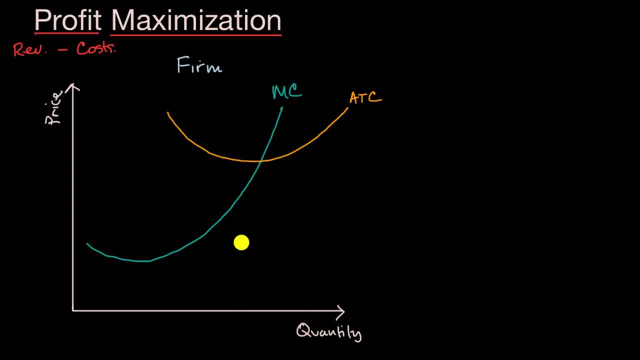 maybe this is a donut company. the incremental amount per donut is going to stay the same, regardless of how much this firm in particular produces. So let's say that the marginal revenue in this industry, in this market, is right over here. 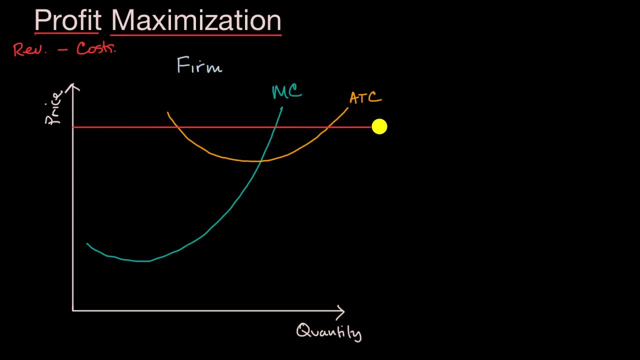 So one way to think about it is: this would be the unit price in that market. So let me put that right over there: marginal revenue, Once again, for every incremental unit. how much revenue are we going to get? So it would just be the price of that unit. 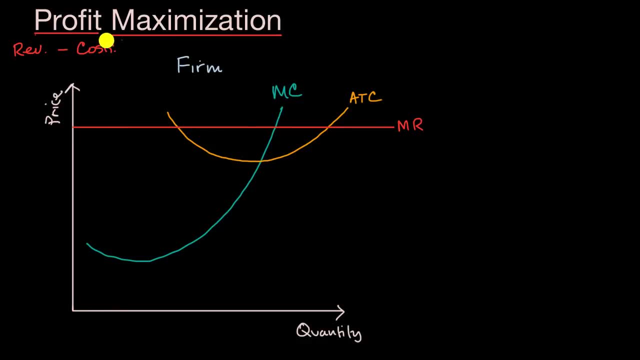 So how much would a rational firm produce in order to maximize its profit If the marginal revenue is higher than the marginal cost? well, that means every incremental unit it produces it's going to bring in some net money into the door, So it's rational for it to do it. 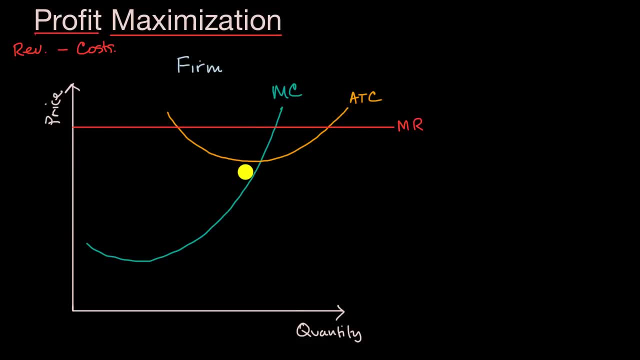 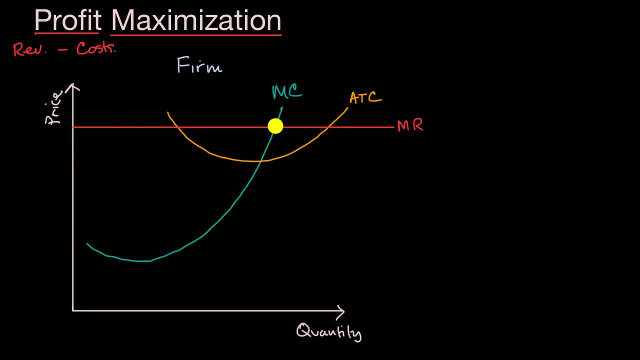 But right at that unit where the marginal cost is equal to the marginal revenue. well, there, on that incremental unit the firm just breaks even, at least on the margin. It might be able to utilize some of its fixed costs a little bit. but then after that point, 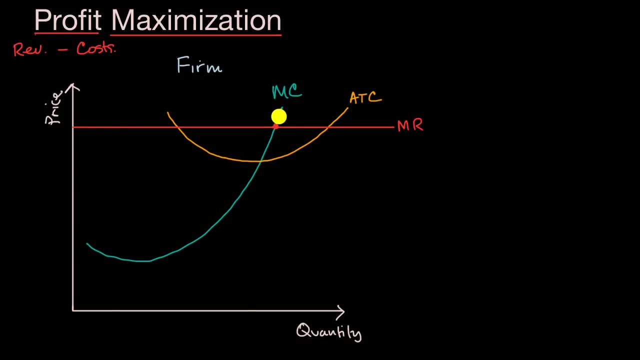 it makes no sense at all for it to keep producing. Why is that? Well, if the marginal cost is higher than the marginal revenue, that would be like saying, hey, I'm gonna sell a donut for a dollar, even though that incremental donut 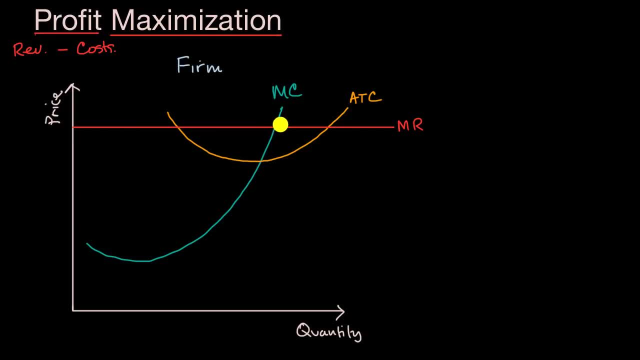 costs me a dollar ten to produce. Well, no rational person, if they wanna maximize their profit, would do that. The firm that's trying to maximize its profit will produce the quantity where marginal cost intersects marginal revenue. It will produce this quantity right over there. 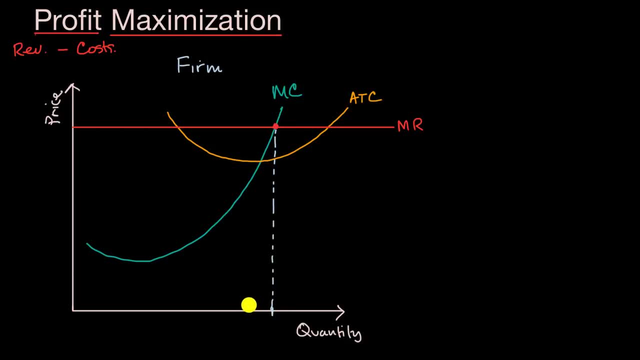 Now, a natural question might be: how much profit will it make from producing that quantity? Well, all you have to do is think about this is the marginal revenue that it gets. and another way you could think about it, because this is constant, it's also going to be.